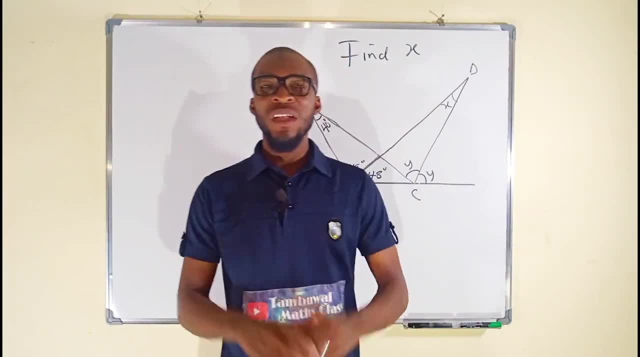 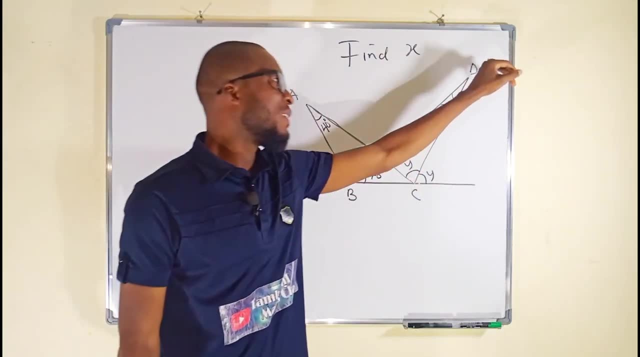 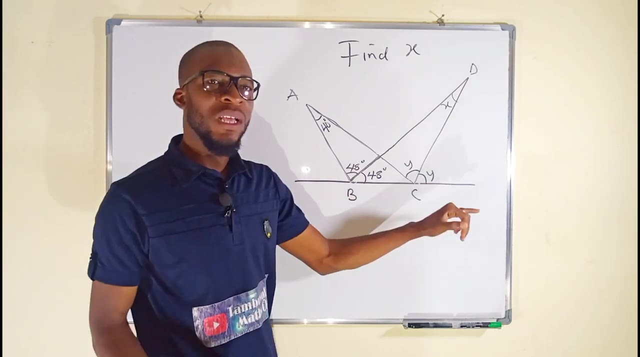 Hello, good morning viewers. In this tutorial we are going to find a solution to this geometry question in which we are asked to find angle D, which X represents. Looking at this diagram, you see we have a straight line in which two other triangles lie on. We have the first triangle, ABC. 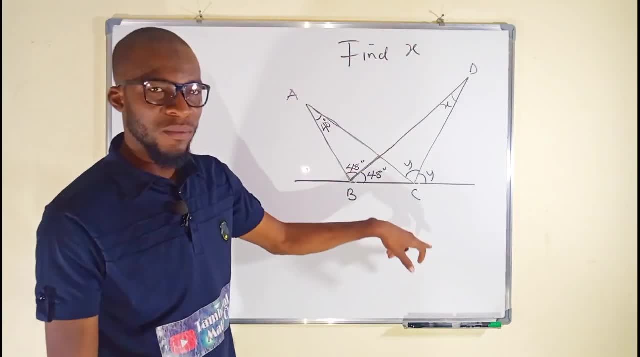 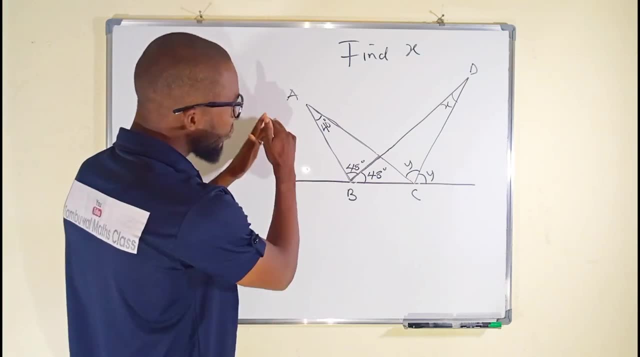 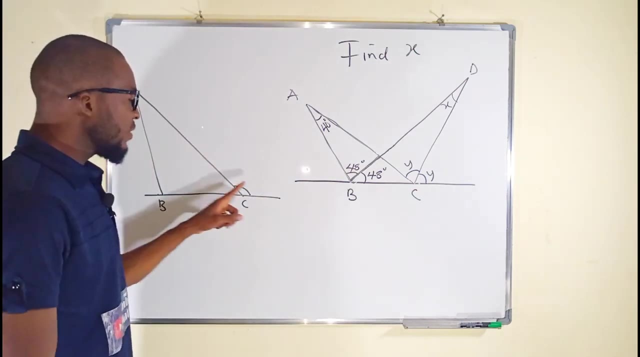 we have the other triangle, DBC, And a smaller triangle is formed between the two triangles. So now let us first of all consider this triangle ABC. Let me make a sketch of that. So this is an exterior angle Of this triangle ABC. you know, all angles inside are said to be. 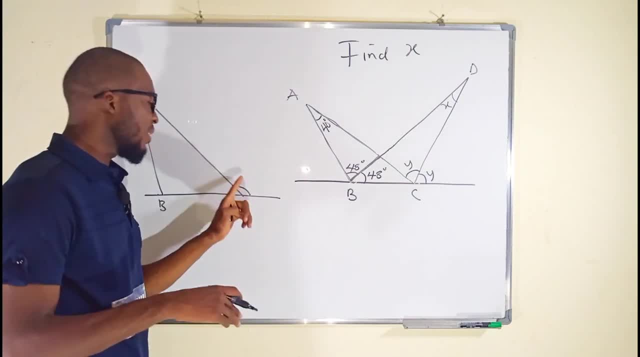 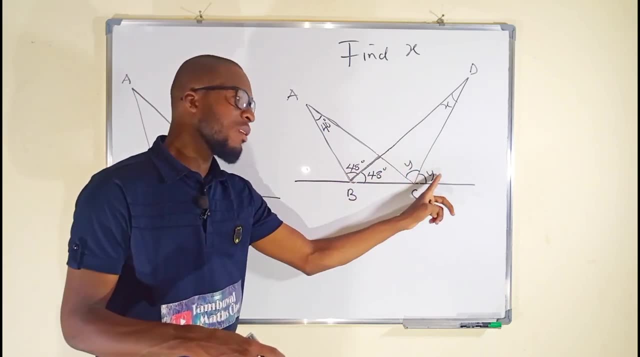 interior and the one outside is said to be exterior, And this angle refers to this Y angle. So this is an exterior angle, So this is an exterior angle, So this is an exterior angle. Y and Y together. Why we have Y and Y? Because this angle and this angle are exactly the same. 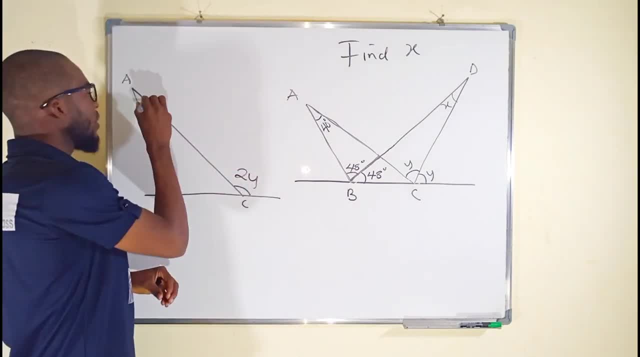 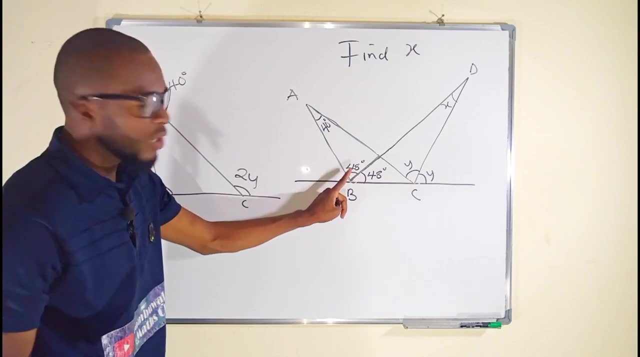 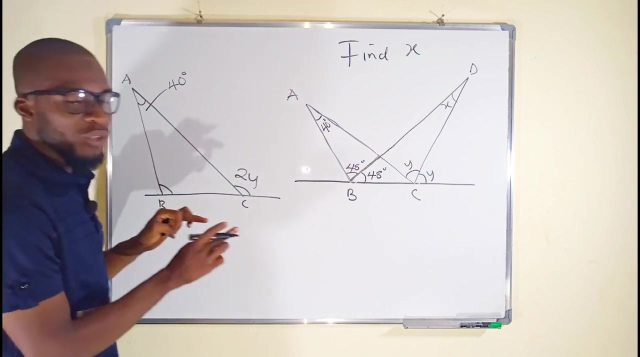 So the two of them make it 2Y. This angle here from the question is 40 degrees And this other one is the combination of these two. You can see we have this 48 and this 48 that comprises of this angle right here. If you join them together, you obtain 96 degrees. 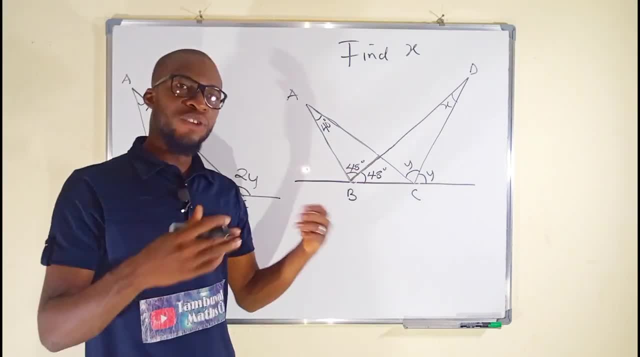 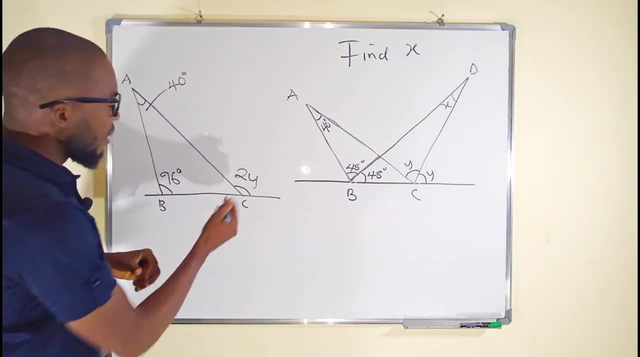 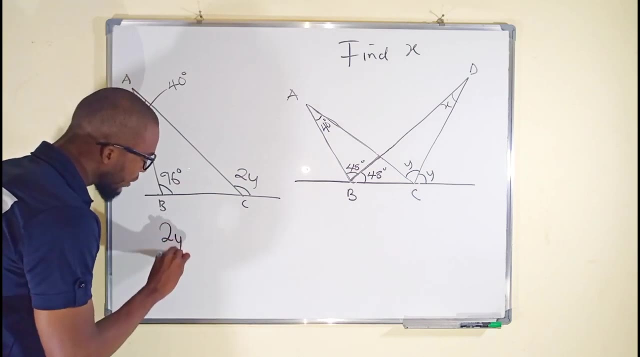 It is one of the laws of a triangle that the exterior angle of a triangle is equal to the sum of the interior opposite angles. This is interior. This is the two opposite angles. If you add them together you must get this 2Y. So we have 2Y to be equal to 40 degrees plus 96 degrees. 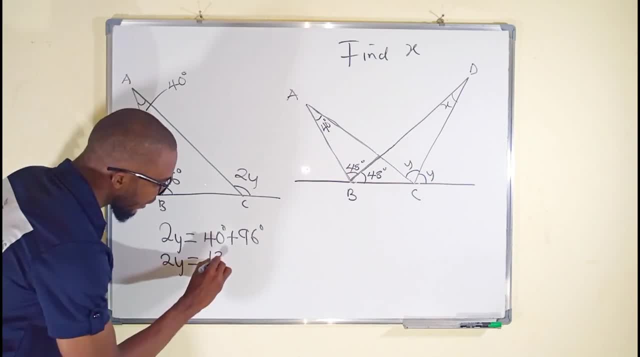 2Y will be equal to 130.. We are looking for the value of Y So we can divide both sides by 2.. Dividing this by 2, we have only Y And, to the right, if you divide 136 by 2, you shall obtain 68 degrees. 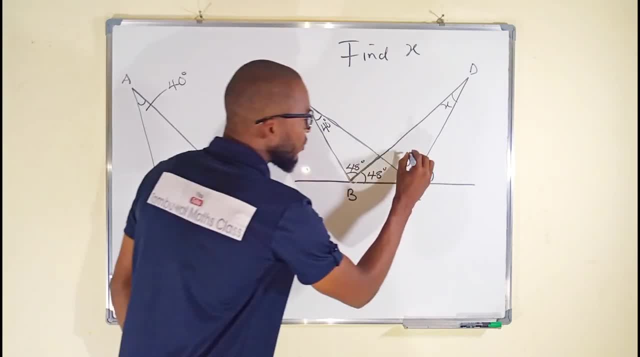 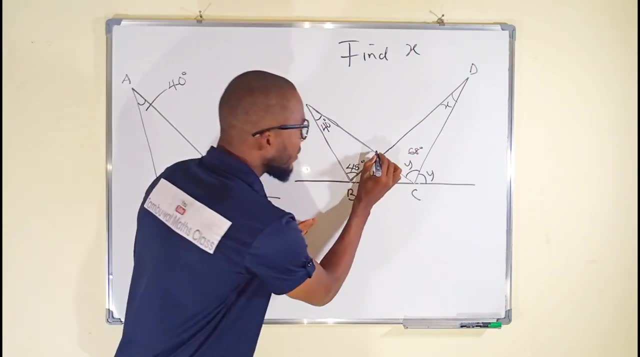 If Y is equal to 68 degrees, we can write this one as 68 degrees. Let me write it very small here. Observe carefully that this is also an exterior angle. This is an exterior angle of this triangle. You see, apart from this big triangle we can form. 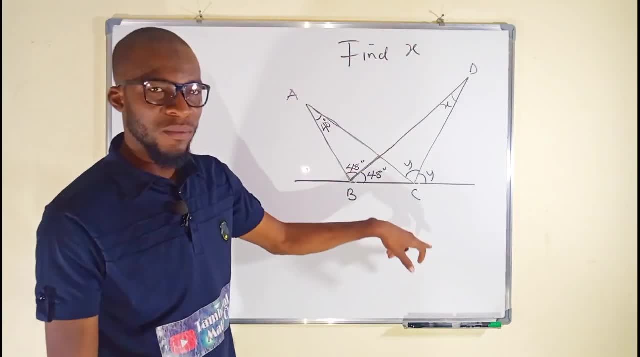 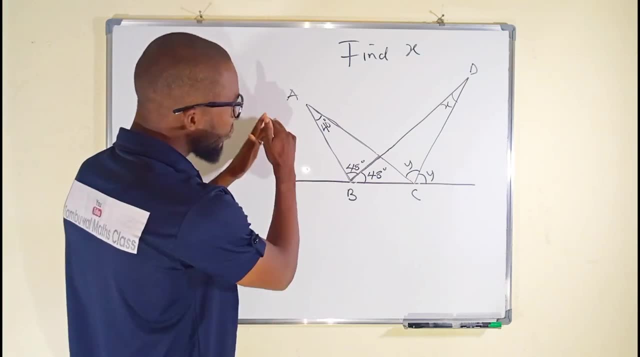 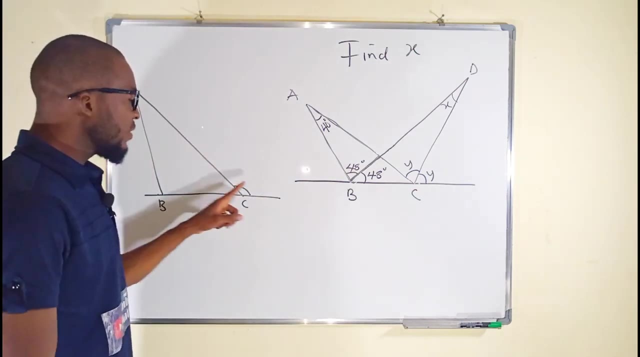 we have the other triangle, DBC, And a smaller triangle is formed between the two triangles. So now let us first of all consider this triangle ABC. Let me make a sketch of that. So this is an exterior angle Of this triangle ABC. you know, all angles inside are said to be. 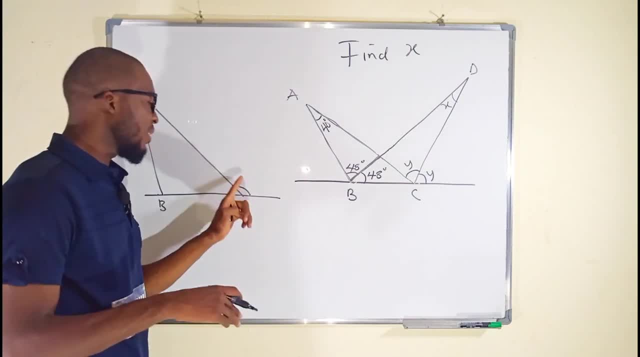 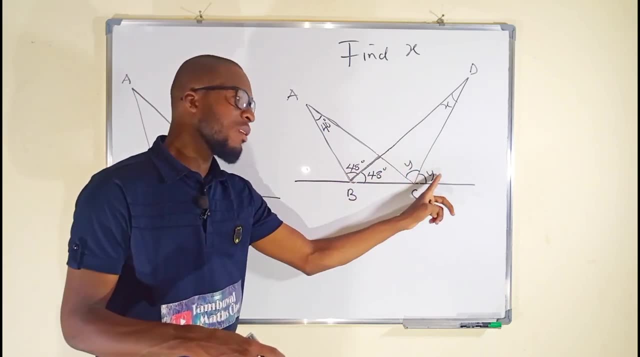 interior and the one outside is said to be exterior, And this angle refers to this Y angle. So this is an exterior angle, So this is an exterior angle, So this is an exterior angle. Y and Y together. Why we have Y and Y? Because this angle and this angle are exactly the same. 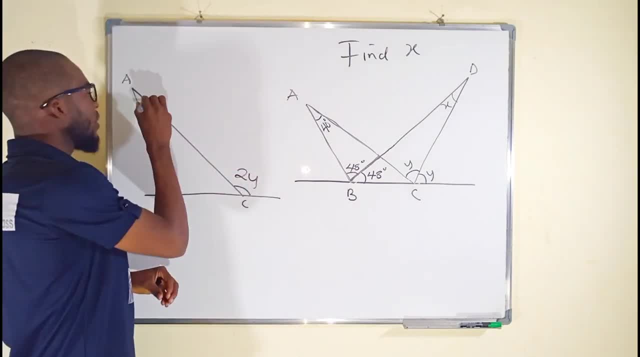 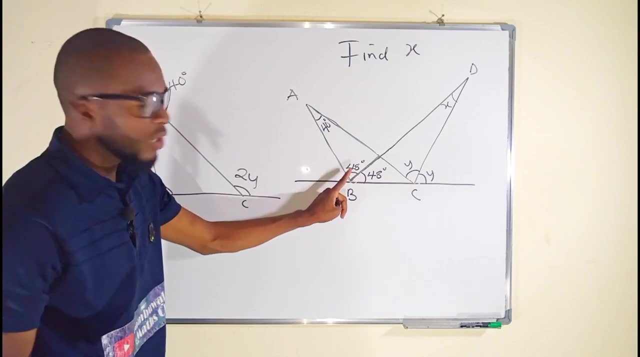 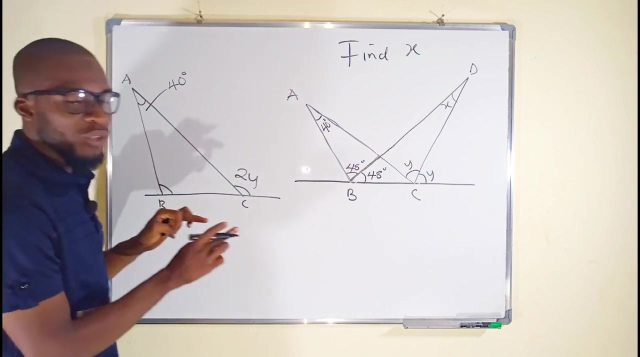 So the two of them make it 2Y. This angle here from the question is 40 degrees And this other one is the combination of these two. You can see we have this 48 and this 48 that comprises of this angle right here. If you join them together, you obtain 96 degrees. 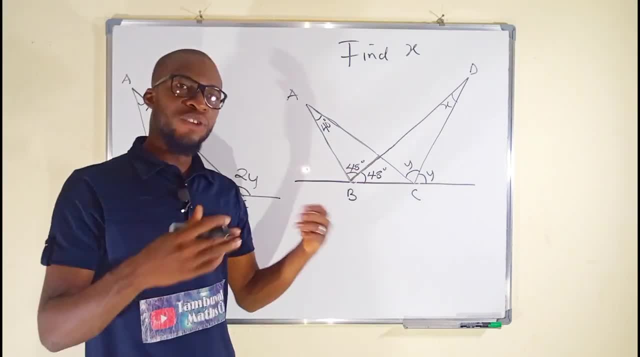 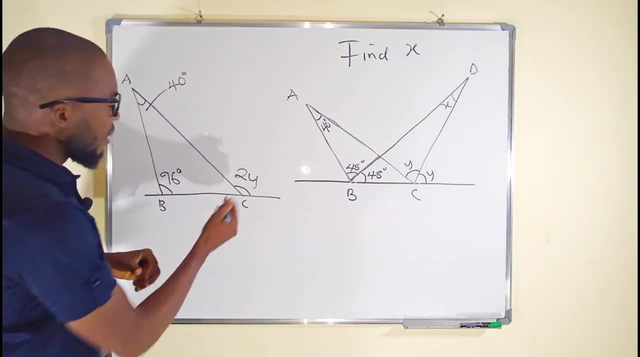 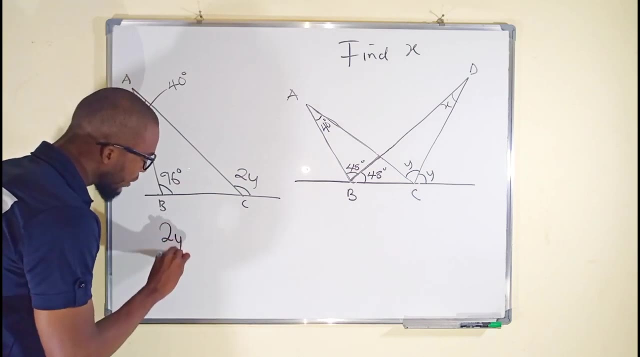 It is one of the laws of a triangle that the exterior angle of a triangle is equal to the sum of the interior opposite angles. This is interior. This is the two opposite angles. If you add them together you must get this 2Y. So we have 2Y to be equal to 40 degrees plus 96 degrees. 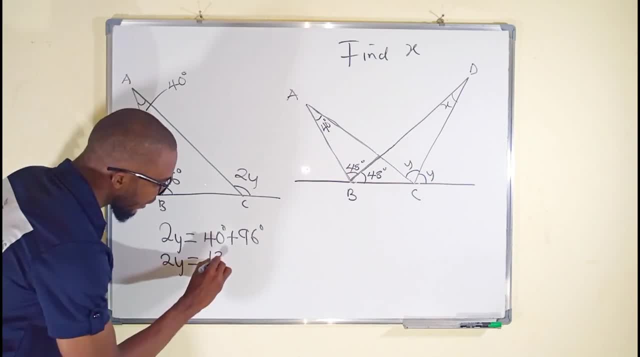 2Y will be equal to 130.. We are looking for the value of Y So we can divide both sides by 2.. Dividing this by 2, we have only Y And, to the right, if you divide 136 by 2, you shall obtain 68 degrees. 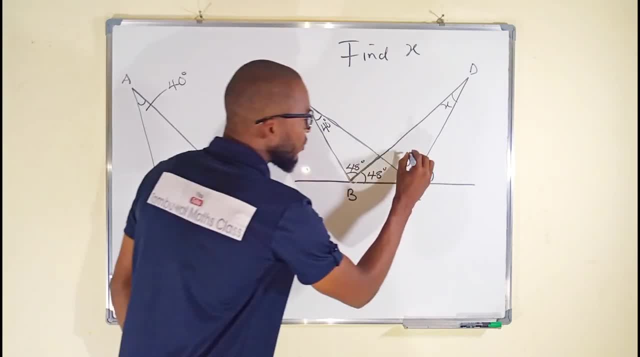 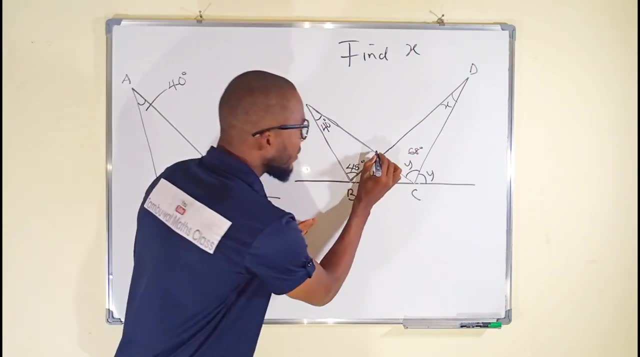 If Y is equal to 68 degrees, we can write this one as 68 degrees. Let me write it very small here. Observe carefully that this is also an exterior angle. This is an exterior angle of this triangle. You see, apart from this big triangle we can form. 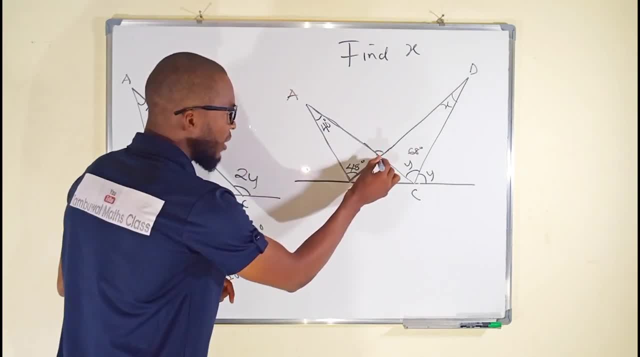 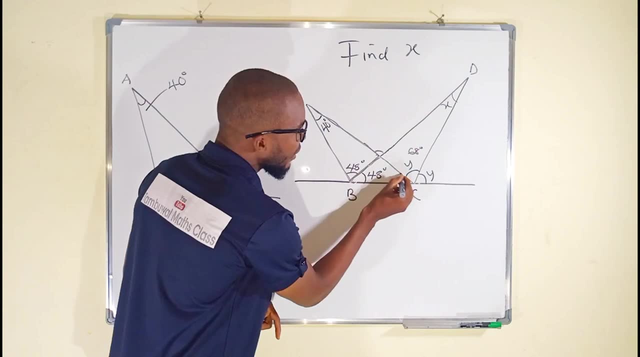 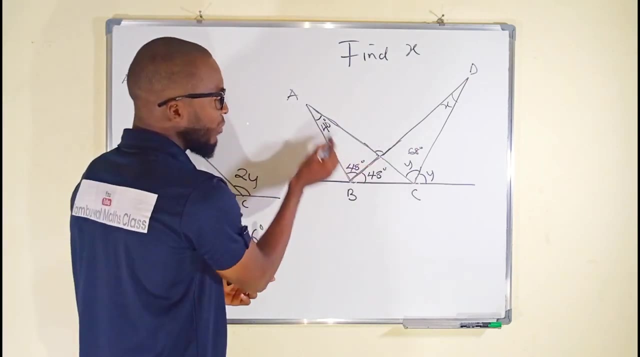 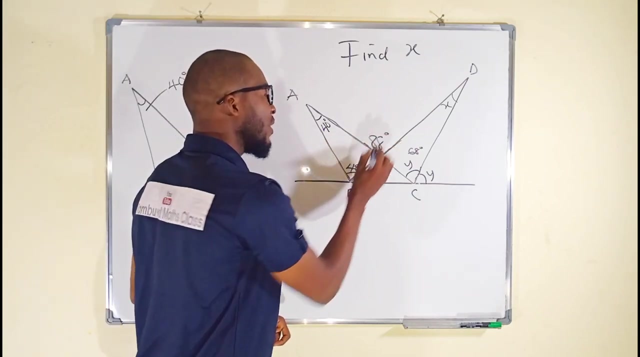 another one here. Look at it here From here upward. This is an exterior angle of this triangle, as well as this other one. Look at it here Upward: The same thing. if you want to find this angle, you can sum this interior opposite angles together: 40,, 48,, making 88. So this angle right.